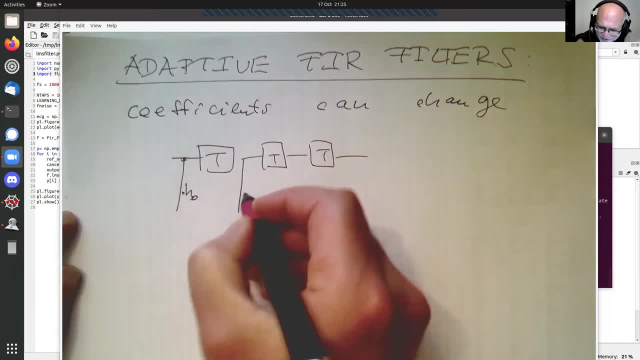 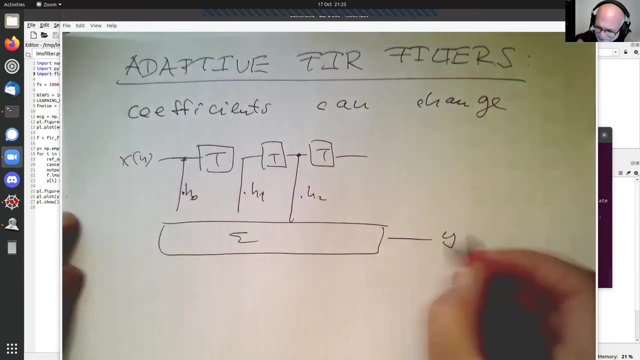 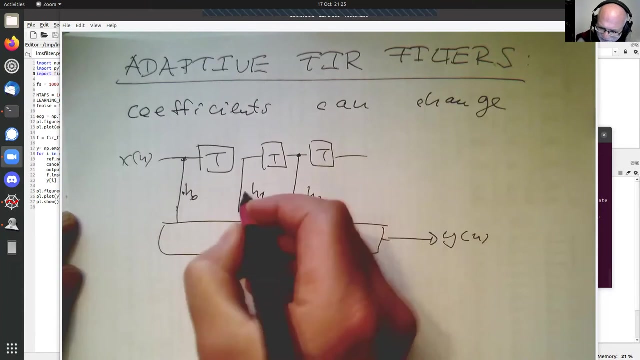 Multiplied by this coefficient, and then multiplied by this coefficient, and multiplied by this coefficient, and then we have an output here. So that's our input: x of n, That's our output y of n. And so here so these coefficients, here. 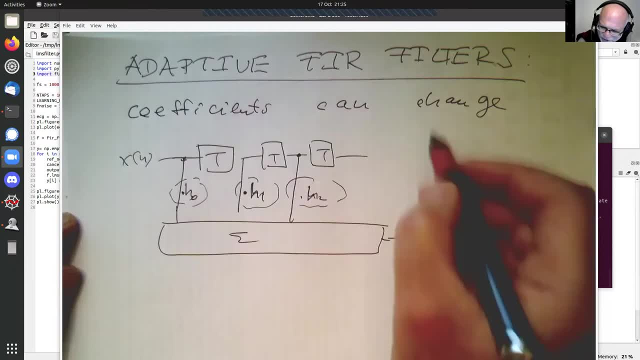 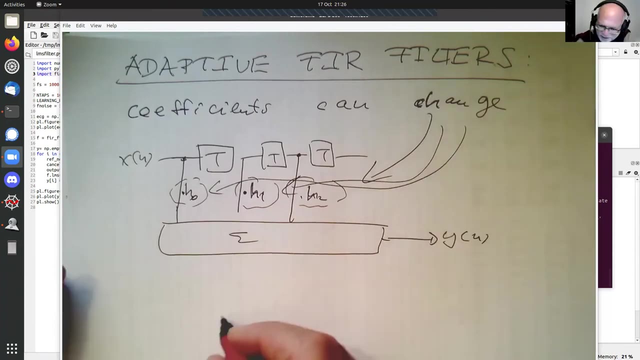 they can now change. So these are now able to change, And so now the question is obviously: how do we change these coefficients, And so why would we do it So? so we need to address this: how to change, And then obviously also: 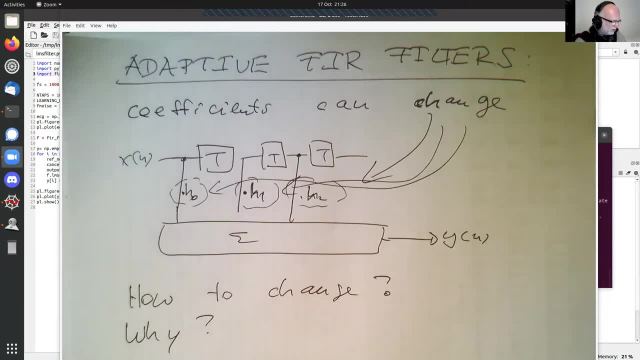 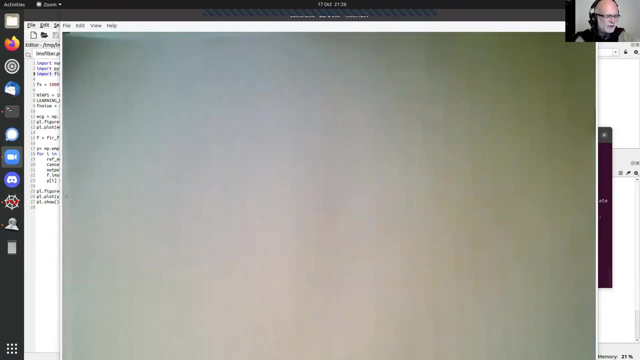 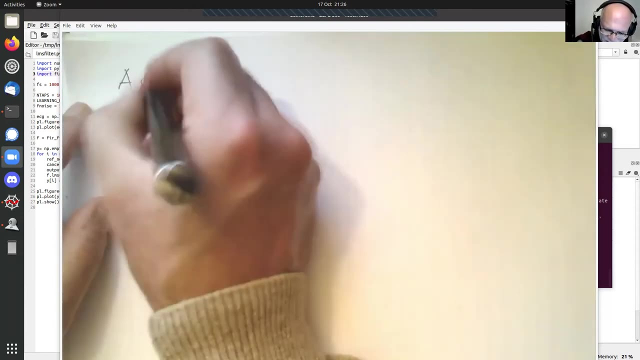 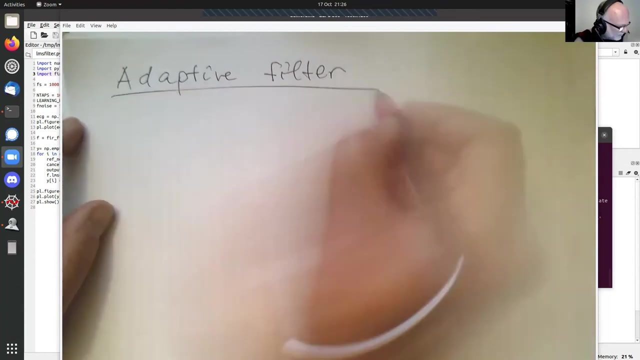 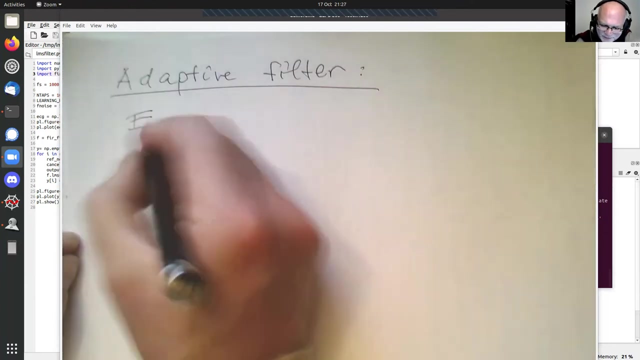 so why would we change coefficients? So that's obviously not directly clear why we would do that anyway, And so let's just find a motivation for this here. So let's just continue with what we did here. We did have the first step of the first step. 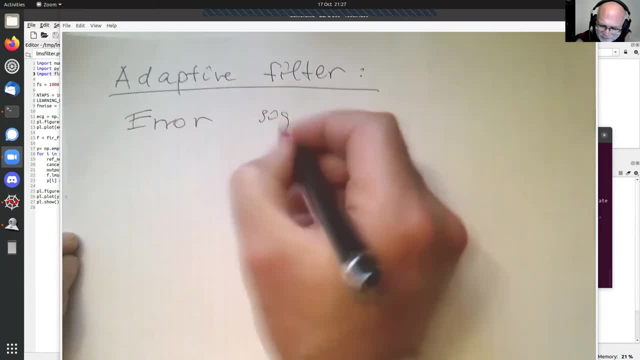 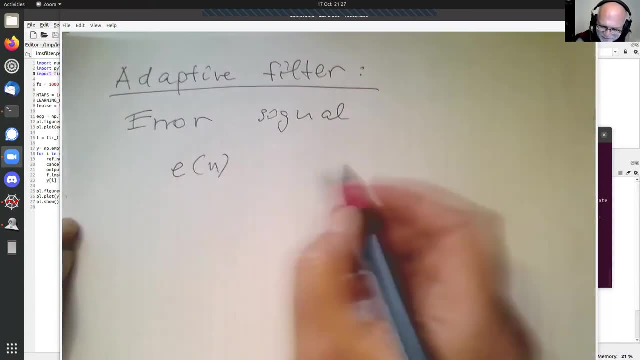 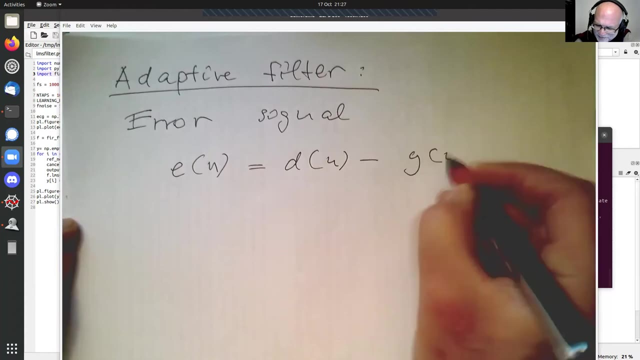 which was to introduce an error signal, And that's what we're going to do here. So let's just go here and let's introduce an error signal. So how do we do that? between a desired state and Y, which is the output. So we have a desired filter output. 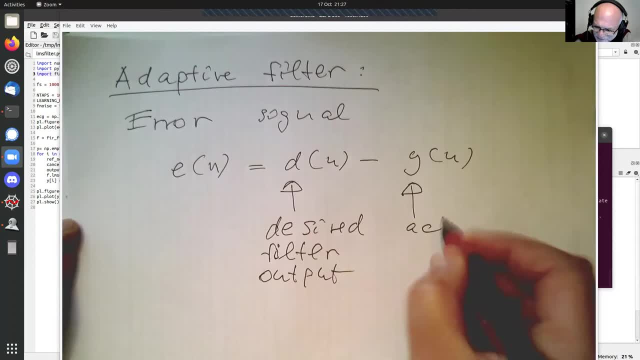 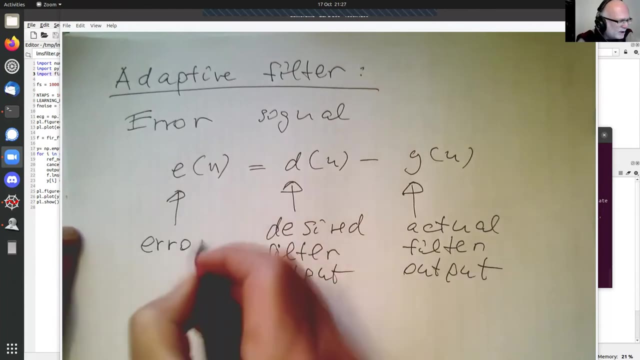 And here we have the actual output, the actual filter, And then we're defining an error signal here. And so what we're doing is, with the error signal is here, with the error signal, with this error signal we tune the FIR filter. 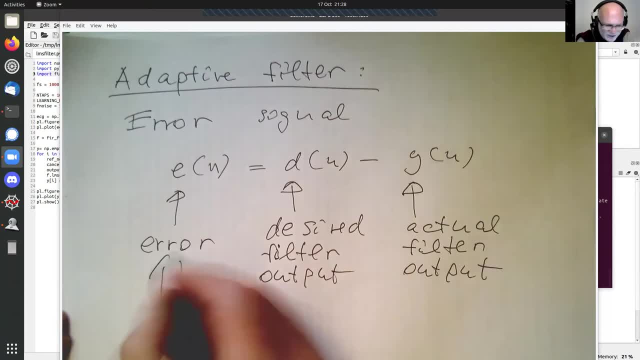 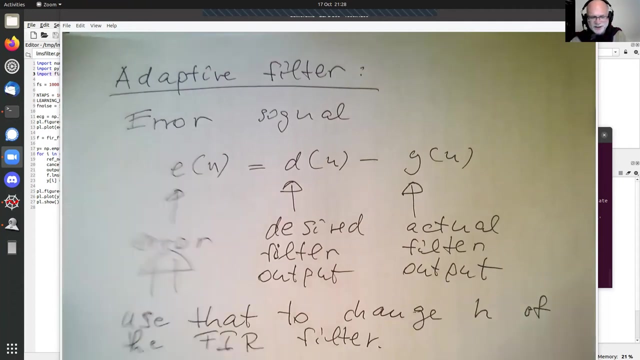 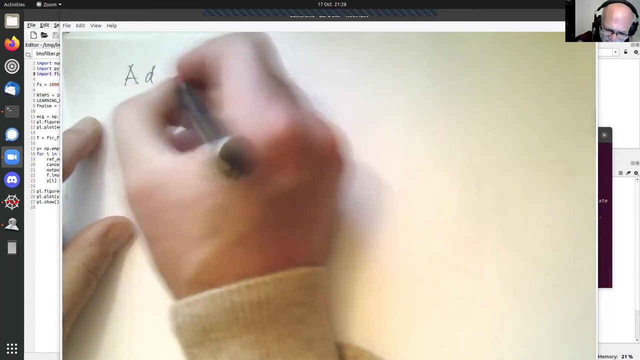 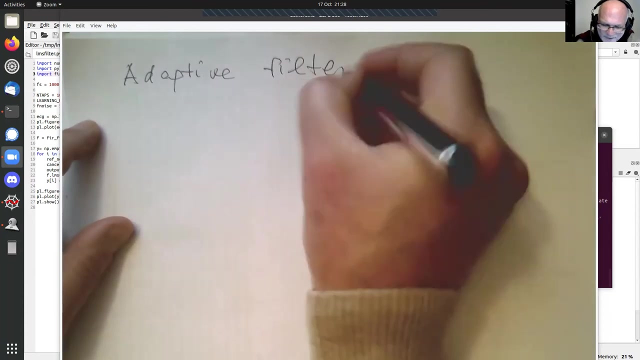 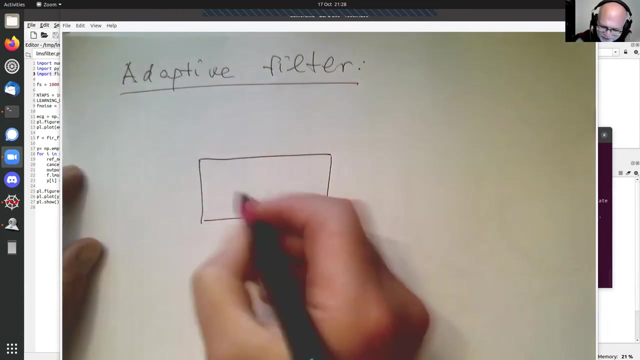 and change the coefficients here. So with that, so use that to to change H of the FIR filter, So we can draw this as a simplified version of this. So, adaptive filter, Let's just draw the FIR filter just here as a box. 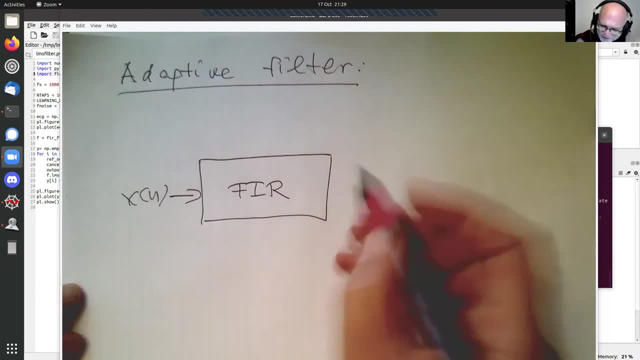 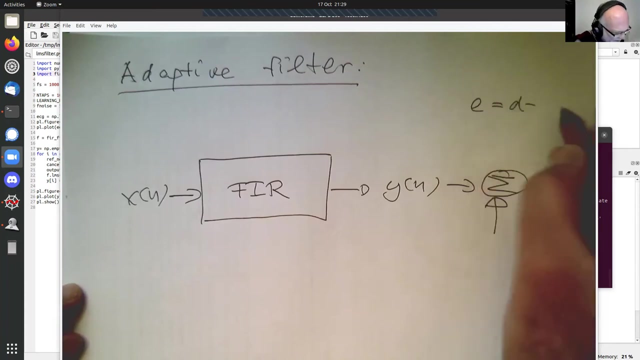 And it gets this X of n And then the output is Y of n, And so now what we're doing is here. so remember the definition. what I had here is e equals to is d minus d minus y, So our error signal. So we have here our d of n and this our y of n. 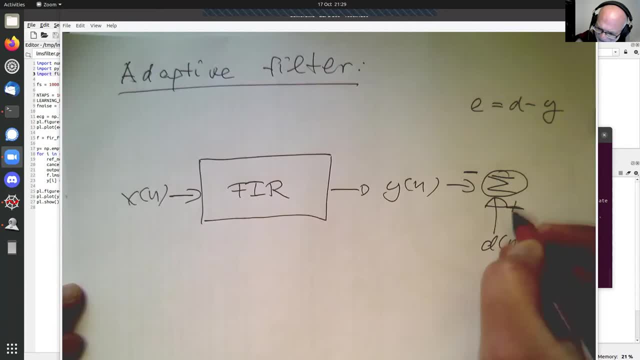 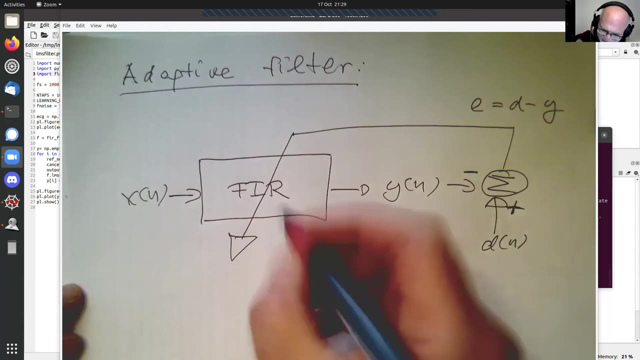 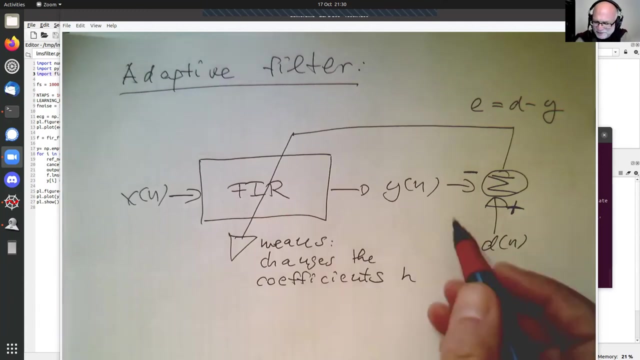 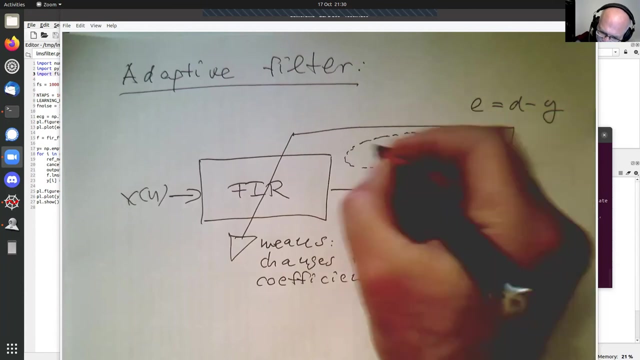 And this is your negative and this is your positive. And then this is here: changing the coefficients of the filter. So this means here changes the coefficients, Coefficients h, And so we have here a negative feedback loop. So like that here, So that's a negative feedback loop. 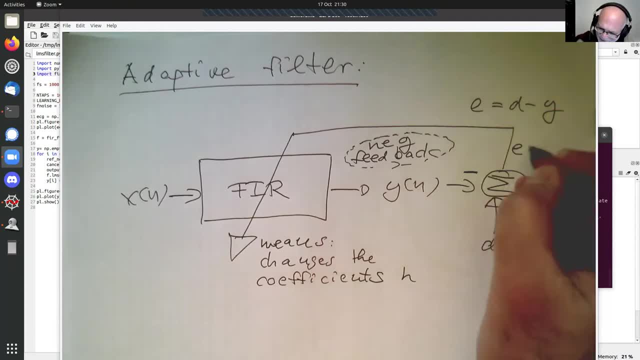 And so the error signal e here, e of n Then, will be changed in the way that at some point it will be zero. And so let's say that the error signal manipulates the FRR filter in the way that y is changing.